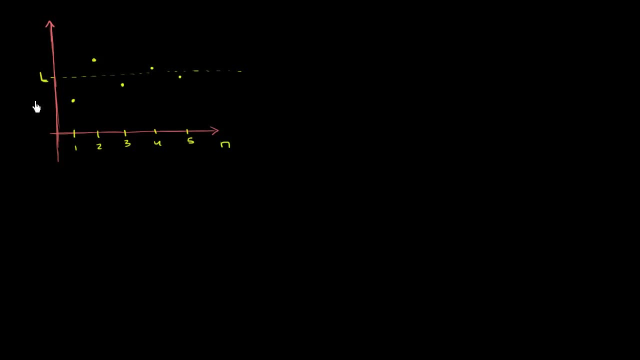 with a definition of what does it really mean to converge to l? So let's say: for any. so we're going to say that you converge to l If for any epsilon greater than 0, for any positive epsilon, you can come up, you can get, or you can there is. 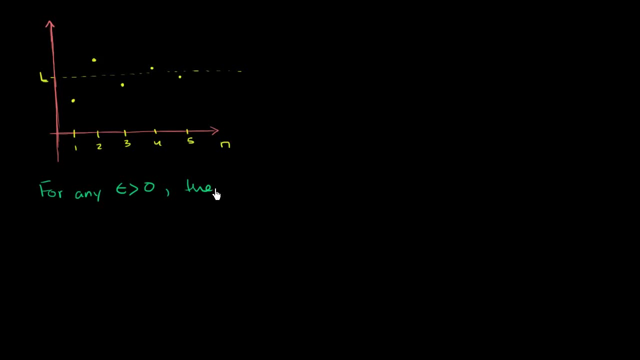 or maybe I'll write it this way: for any positive epsilon there is a positive epsilon, There is a positive m, capital M, such that if lowercase n is greater than capital M, then the distance between a sub n and our limit this l right over here. 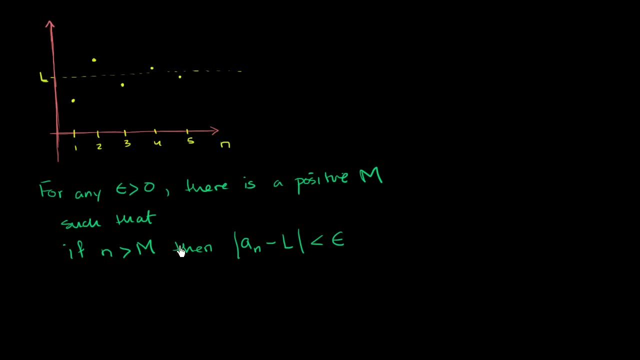 the distance between those two points is less than epsilon. If you can do this for any epsilon, for any epsilon greater than 0, there is a positive m, such that if n is greater than m, then the distance between a sub n and our limit 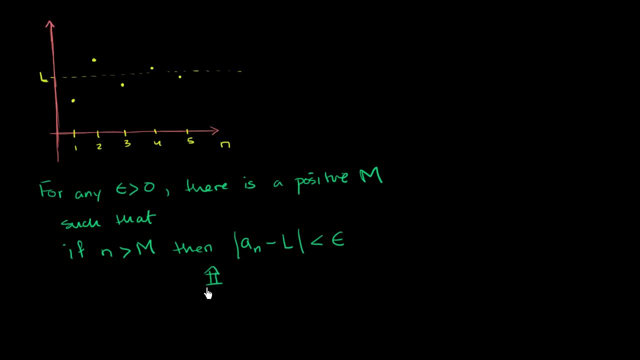 is less than epsilon, Then we can say that the limit of a sub n, as n approaches infinity is equal to l, And we can say that a sub n converges to l. So let's parse this So here I was making the claim that a sub n is approaching. 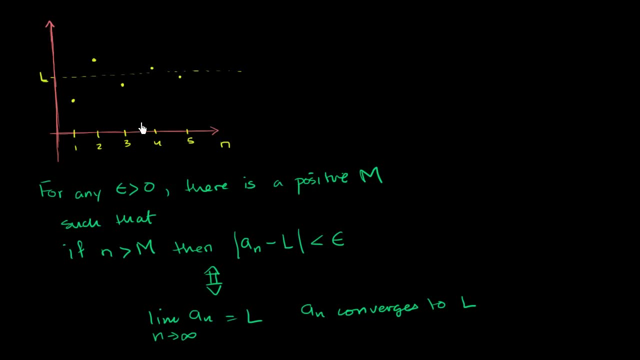 this l right over here. I tried to draw it as a horizontal line. This definition of what it means to converge for a sequence to converge says: look for any epsilon greater than 0, so let me pick an epsilon greater than 0.. 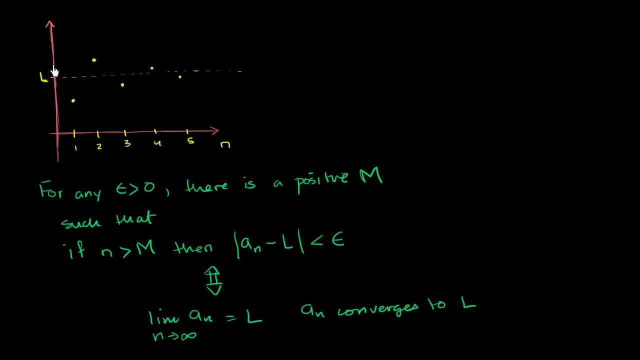 So I'm going to go to l plus epsilon. Actually, let me do it right over here. Let's say this is l plus epsilon, And let's say this is right here: This is l minus epsilon. So let me draw those two bounds right over here. 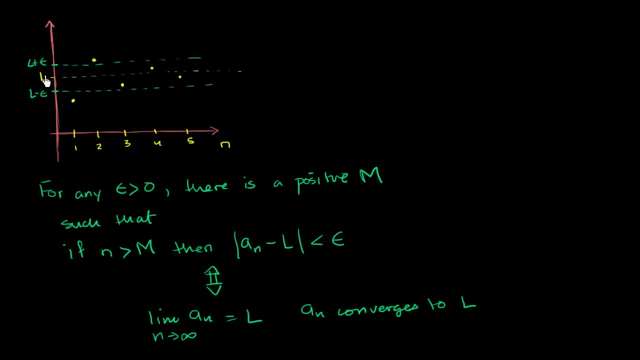 And so I picked an epsilon here. So for any arbitrary positive epsilon I pick, we can find a positive m, so that as long as so let's say that that is our m right over there. so that as long as our n is greater than our m,